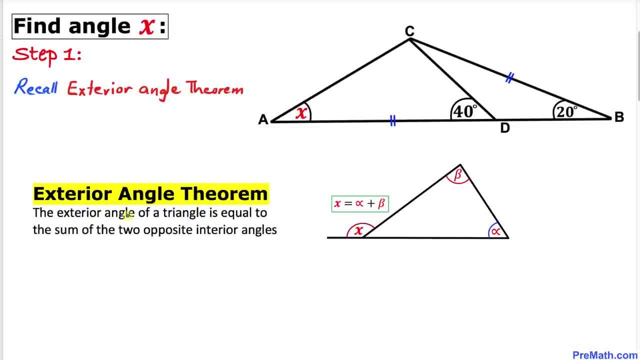 and here's our exterior angle theorem. The exterior angle of a triangle is equal to the sum of two opposite interior angles. In our case, over here, this is our exterior angle and this is going to be equal to the sum of these two opposite interior angles: alpha and beta. Now let's focus on our this triangle BCD. We can see: 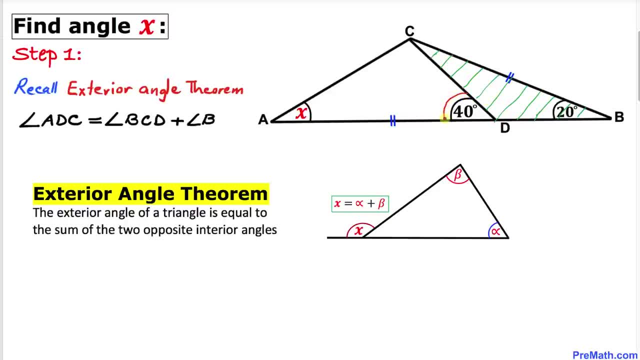 that this 40 degrees is our exterior angle and this is going to be equal to the sum of these two opposite interior angle: this angle and this angle. so therefore, this angle has got to be 20 degrees. so therefore, our angle BCD turns out to be 20 degrees, and now we know that these two angles are equal. so 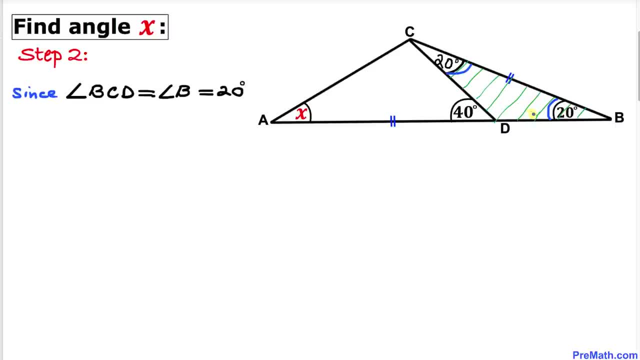 that means this triangle is an isosceles triangle, so therefore this side is going to be equal to this side, therefore this BD side equal to CD. and here's our next step. let's observe this one: we know that this side length AD equal to this side length BC. therefore, we moved this triangle BCD. 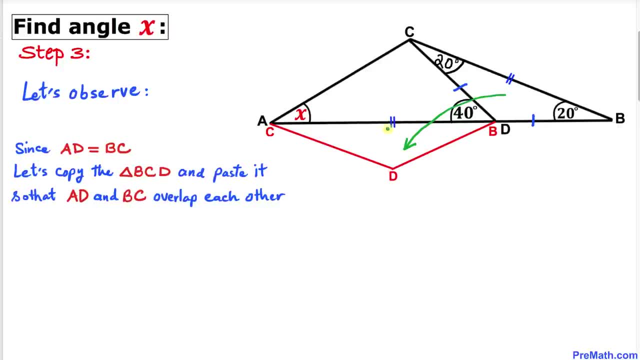 right up here, such that this side length, AD and BC, they overlap each other and, moreover, these, our BCD Worth column, are equal to 20 degrees. Now, a little distinction about this is that this is our mirror Skin. 1 angle is, firstly, ropes. that has been converted into these red BC and D, As you can see in this figure, and, moreover, these angles are: 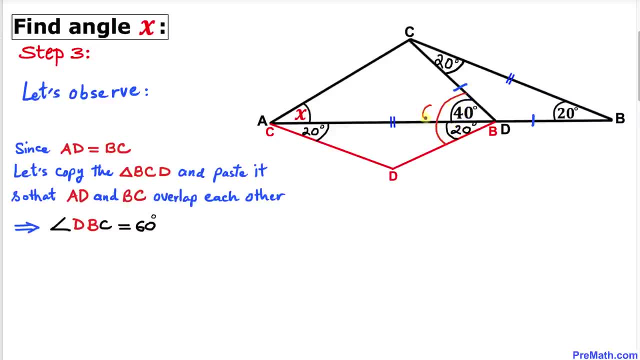 going to be same as well: 20 degrees and this one, and 20 degrees, this one as well, since these two triangles are identical. so therefore, this whole angle DBC is quick-winner, I'm sorry, see you later. to be: 20 plus 40 is going to become 60 degrees, and here's our next step. we know that these two 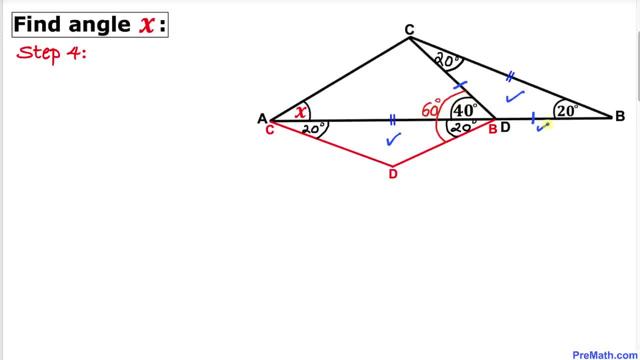 triangles are identical and we know that these two sides are equal, so that means this side is going to be equal to this side as well. and now let's go ahead and connect these two points. we're going to connect this point c and this red point d, and here's our much nicer looking diagram and as a 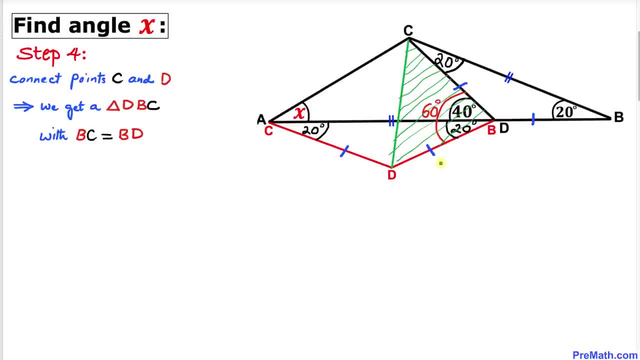 result we get this triangle: dbc with this side is equal to this side length. and now, since this is an isosceles triangle, since these two sides are equal in length and this angle is 60 degrees, so therefore these two angles have got to be equal as well, and this angle is going to be 60 degrees. and this angle is going to be 60 degrees. 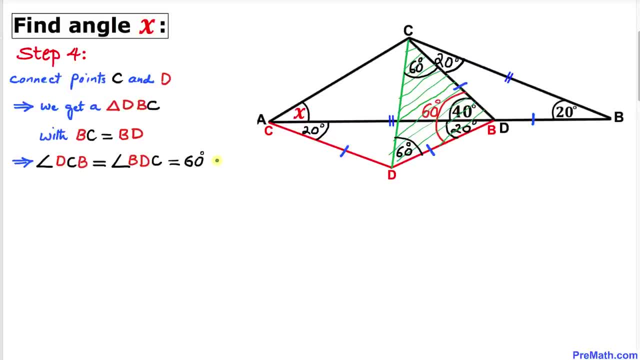 as well. so therefore, we got these two angles equal to 60 degrees as well. so therefore, we conclude that this triangle is an equilateral triangle, since all these angles are 60 degrees. so that means this side is going to be equal to. this side is going to be equal to. this side is going to be. 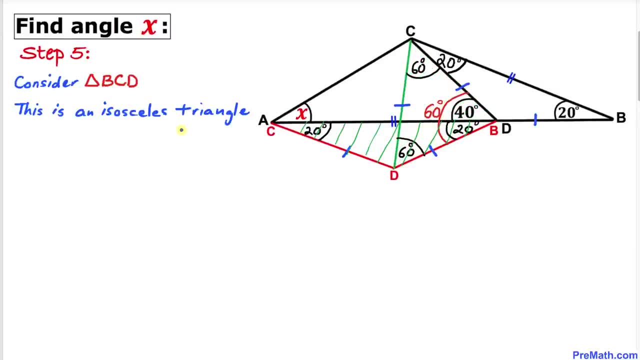 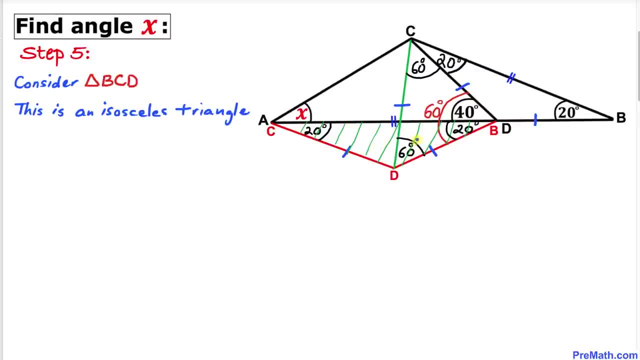 know that the angle sum in this triangle is going to be 180 degrees. if this angle is 20 degrees, this angle is 20 degrees, so that means this angle has got to be 140 degrees. therefore, our angle BDC turns out to be 140 degrees. and now 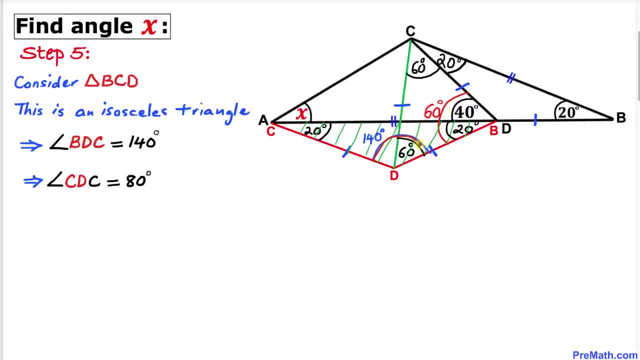 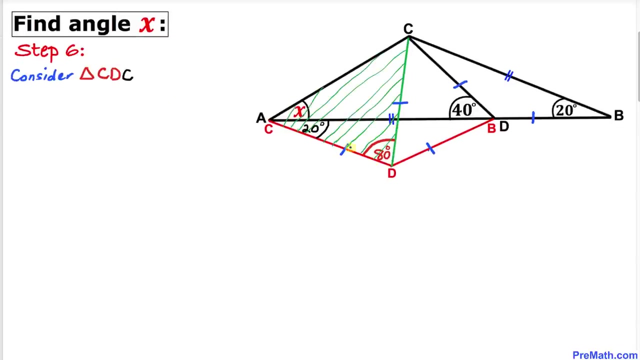 we can see that this whole angle is 140 degrees and this angle is 60 degrees. so this angle has got to be 140 minus 60 is going to be 80 degrees. so therefore, our this angle, CD see, turns out to be 80 degrees. and here's our final step. let's focus on 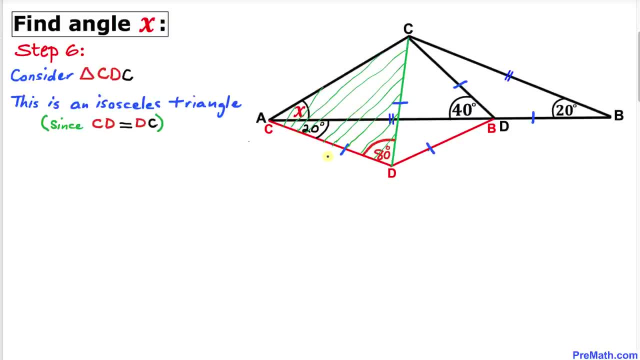 this triangle, CDC, and we know that this is an isosceles triangle, since this side length equal to this side length. so therefore, this angle has got to be equal to this angle and we know that this angle is, this whole angle, is X plus 20 degrees. so that means this angle has got to be X plus 20 degrees as well. 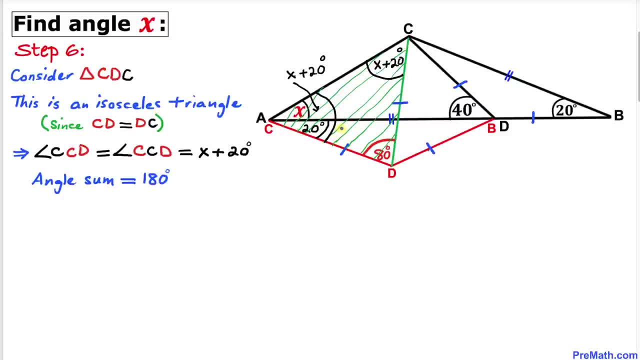 and we also know that the angle sum of any triangle is 180 degrees. so that means, in this triangle, sum of all these three angles, this angle, this angle and this angle must add up to 180 degrees. let's go ahead and add up all these angles. I'm going to add up all these angles. I'm going to add up all these angles, I'm going to. 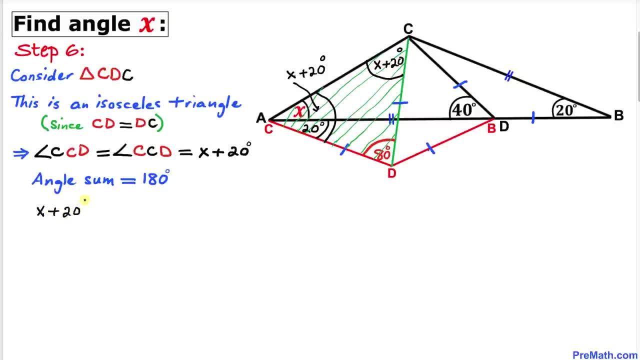 write down: X plus 20 degrees, first angle, and likewise X plus 20 degrees, our next angle, and plus 80 degrees has got to be equal to 180 degrees. and now let's go ahead and combine the like terms: is X plus X is going to give us 2x, and let's 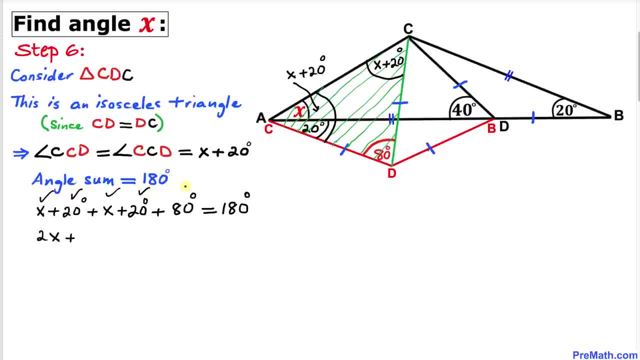 combine these angles- 20 degrees plus 20 degrees plus 80 degrees- that is going to give us 120 degrees, equals to 180 degrees. and now let's go ahead and subtract 120 degrees from both sides and we can see this: positive 120 degrees and negative 120 degrees. they cancel each other out. so we ended up with 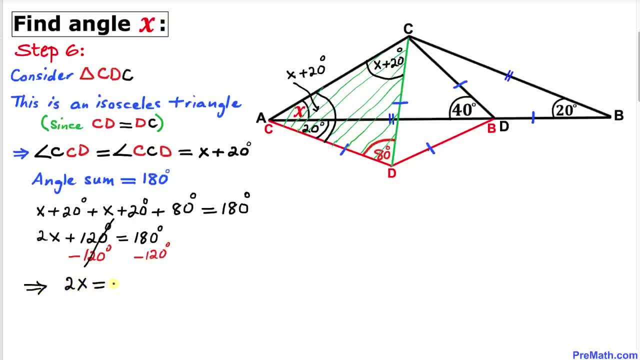 2x, equal to on the right hand side. that is going to give us 60 degrees. let's go ahead and divide both side by 2 to isolate x. this 2 and 2 is gone, so that means our x angle turns out to be 30 degrees. so that means this angle turns out to be 30 degrees. 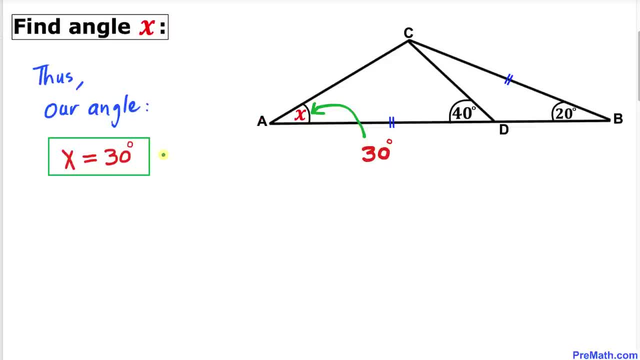 thus, after all these multiple steps, our angle turns out to be 30 degrees, and that's our final answer. thanks for watching and please don't forget to subscribe to my channel for more exciting videos. bye.